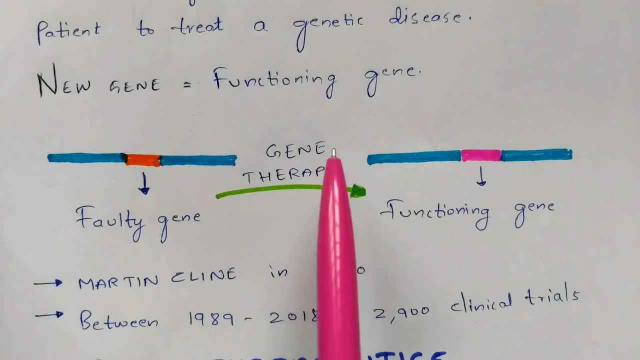 are going to replace with functioning gene, then the process, then the process will be done in such a way that he will not be suffered with this genetic disorder anymore in his life, because he is completely cured by the process of gene therapy. right, So you are going to remove this faulty gene. 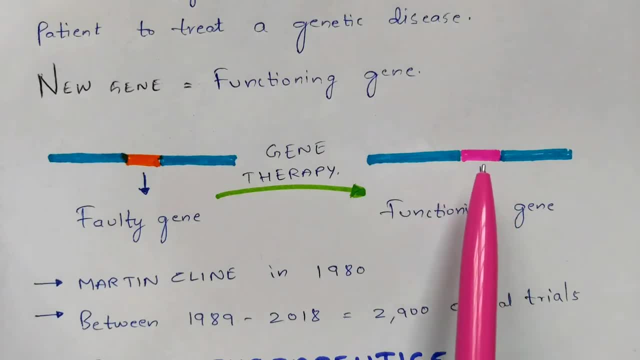 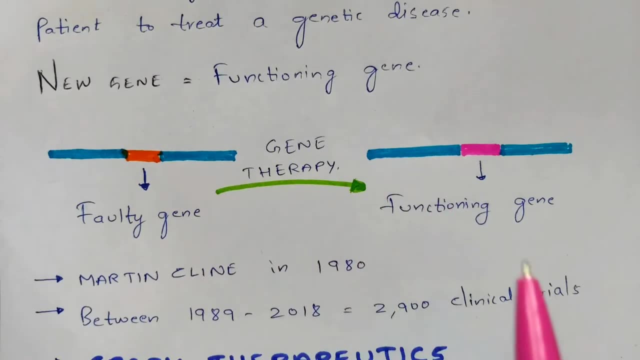 and then you are going to insert the functioning gene in the place of the nucleotide, right? So this process is called as gene therapy. Now you have understood about this gene therapy, right? So this gene therapy process was initially started by a scientist called as Martin Klein in the year of. 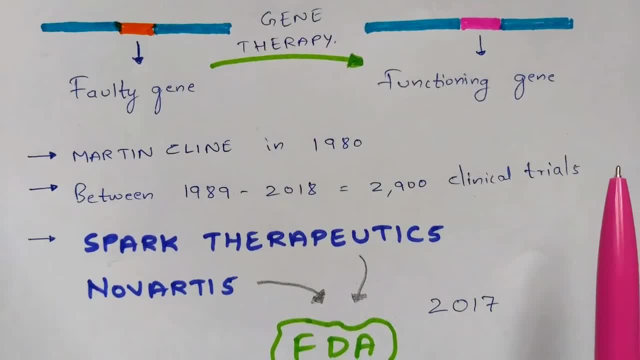 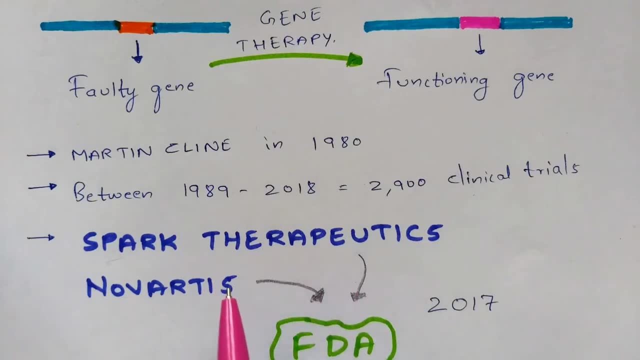 1980. So between the year of 1989 to 2018, there are 2,900 clinical trials which has been done on this gene therapy right and then later two agencies- I mean not agencies like a companies- two companies called as Spark Therapeutics. 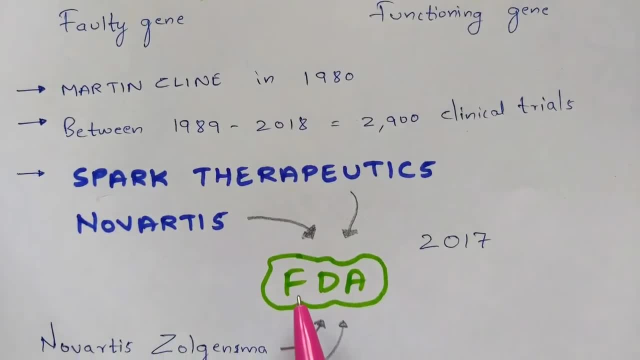 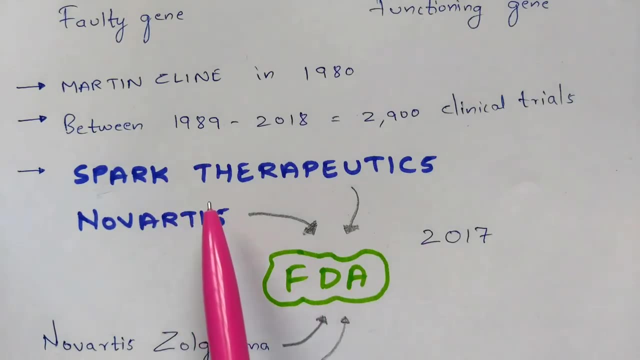 and Novartis are approved by FDA. right, They are approved by FDA in the year of 2017.. So this: both are the companies where they perform this gene therapy process, okay, and hence they are approved by the FDA. So there is no doubt the process of this gene therapy will be done good in this both. 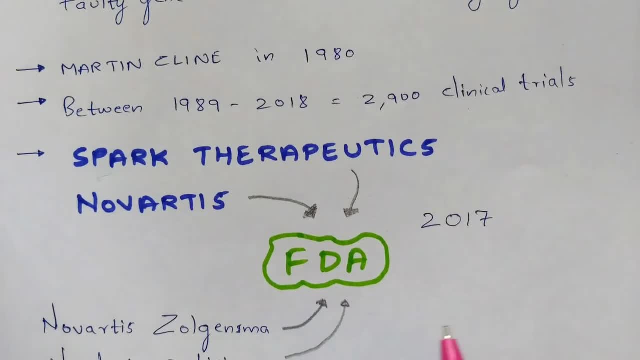 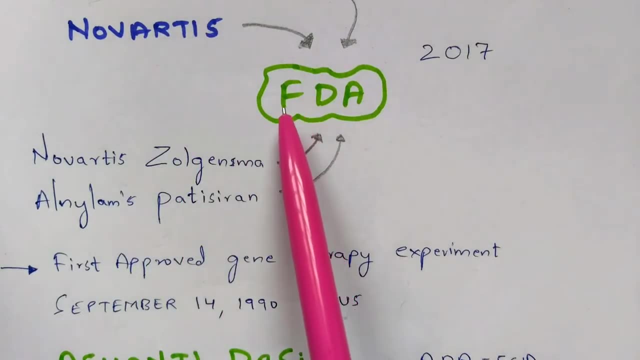 organizations. Okay, so not only this. in the same year of 2017, there are two drugs which are introduced and which are, you know, authorized and approved by FDA itself in order to cure this, you know, genetic disorders and will be useful for this process of gene therapy. So what are those? 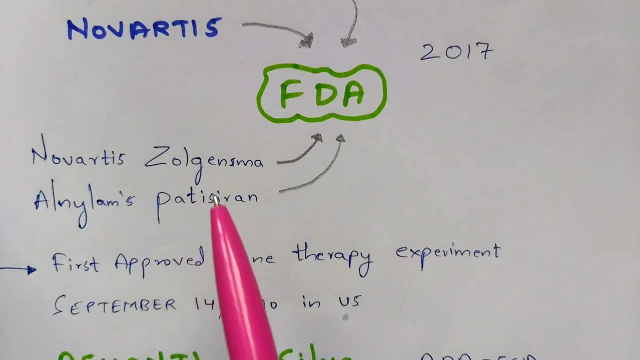 two drugs. They are Novartis and Zolgensma, and another drug is Genesine. Now the second drug is anilines paticerin. so these are the both drugs which are approved by fda in the year of 2017. 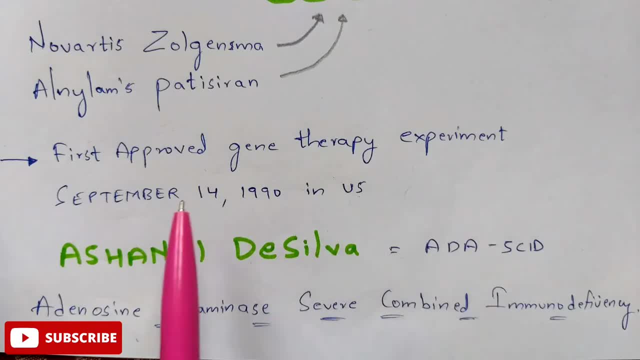 itself. so the first approved gene therapy experiment was done in the year of 1990, on september 14, in united states on a patient called ashanti de silva. so she is a patient who is four years old and she is suffering from ads kit. so ads kit is a genetic disorder which is abbreviated as: 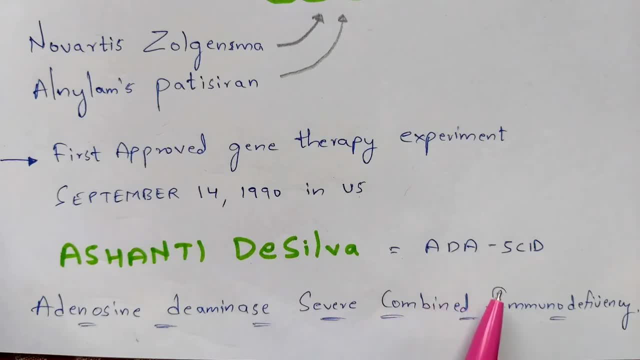 adenosine d minus severe combined immunodeficiency. so she is suffering with this genetic disorder. so in order to cure this genetic disorder, they performed this gene therapy process of experiment, which is approved, which is approved in the year of 1990, on a patient, ashanti de silva. 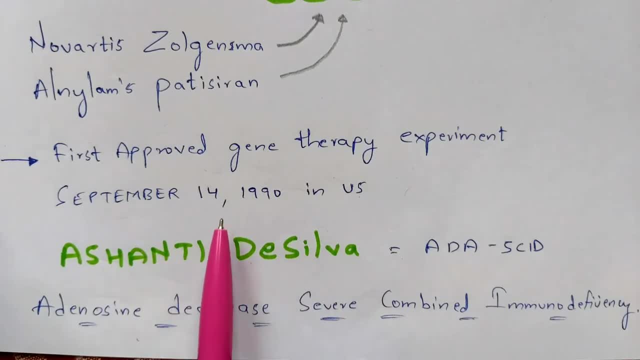 right in united states. so the experiment has been succeeded and she is cured with this genetic disorder. so now let us see clearly about this gene therapy. so till now, what have i explained you is nothing but the introduction about this gene therapy, and now i am going to explain the type of gene therapies and a prosthesis in gene therapy. okay, so listen. 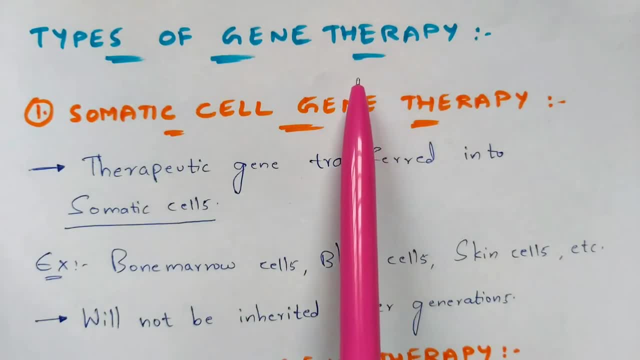 properly. so now let us discuss about types of gene therapy. so there are two types of gene therapies. they are somatic cell gene therapy and germline gene therapy. so firstly let us discuss about somatic cell gene therapy. so the therapeutic gene will be transferred into somatic cells, hence it is 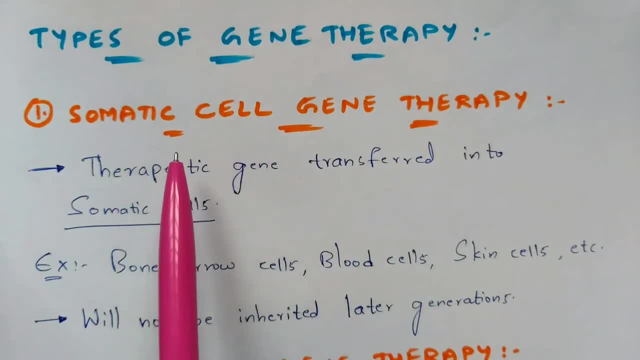 called as somatic cell gene therapy. so what do you mean by this therapeutic gene? so previous, i have said you right, the faulty gene will be replaced by the functioning gene, right, and that functioning gene is called as therapeutic gene, so that therapeutic gene will be transferred into. 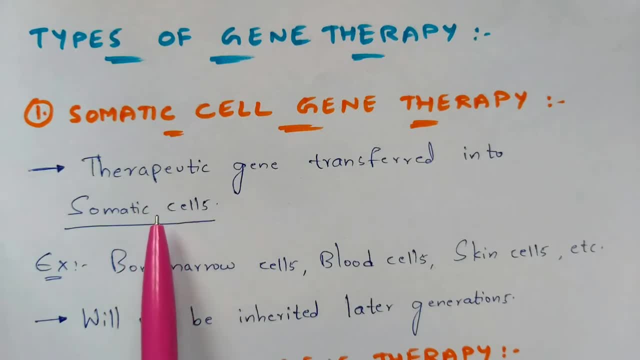 somatic cells of the human being. i mean that patient. hence this process is called as somatic cell gene therapy. so the best examples which we can say are- i mean the best examples of the somatic cells which we can say are bone marrow cells, blood cells, skin cells, etc. i mean the 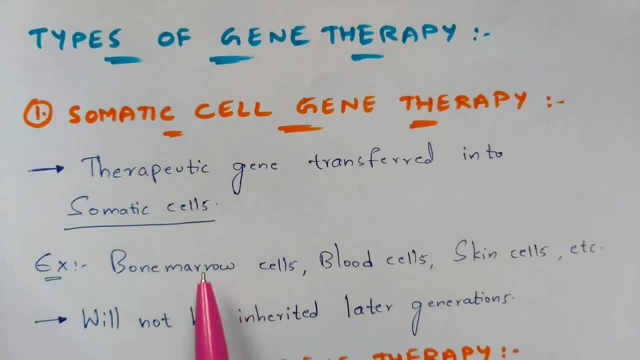 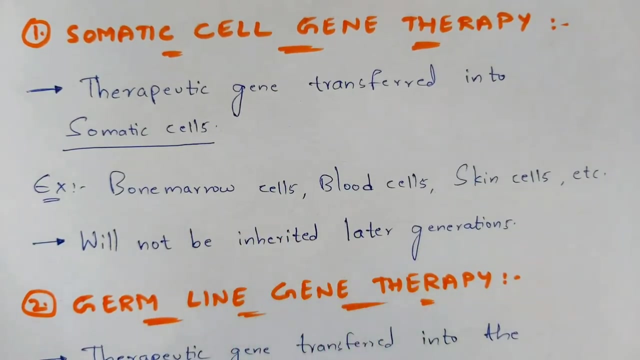 therapeutic gene or the functioning gene will be transferred into these cells. they will choose one particular cell and they will be transferred into the cells right. and one more important thing which people have to remember regarding this somatic cell gene therapy is it will not be inherited into later generations. so now this person, this patient, will 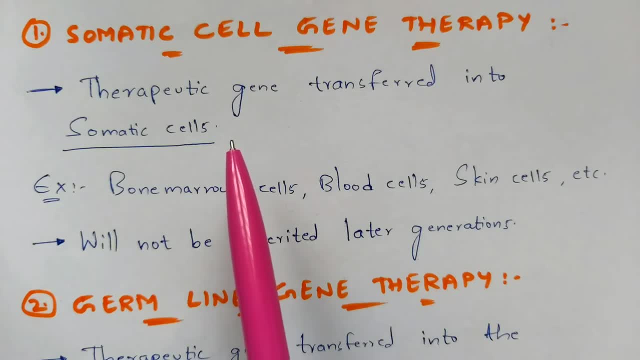 be cured by this process of gene therapy, but if there is no guarantee that this disease will be passed to the future generations, it may be passed or it may not be passed. i mean, this is just a temporary purpose, where only this disease will be passed to the future generations. so this is just a 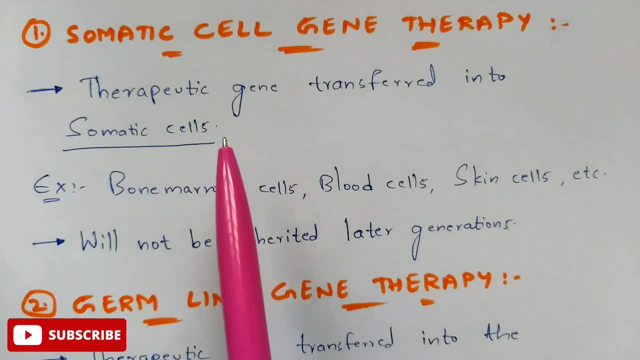 patient can be cured by this disease, there is no guarantee that the disease can be passed to the future generations, i mean to his offspring, for children, right. so it will not be inherited into later generations. so now coming to the second one, which is germline gene therapy. here, the therapeutic 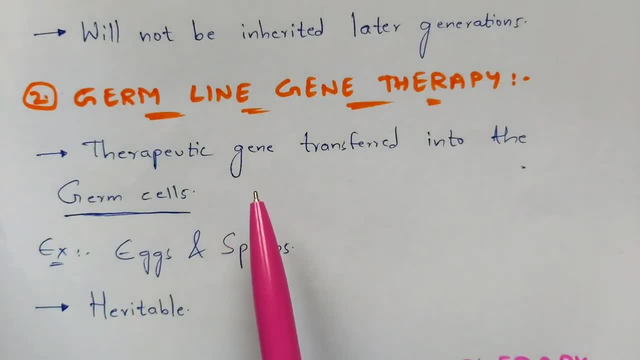 gene, therapeutic gene in the sense which i have said, you right, which is also called as functioning gene, which will be you know where. the faulty gene will be replaced by that functioning gene. so that is called as therapeutic gene and it will be transferred into the germ cells. 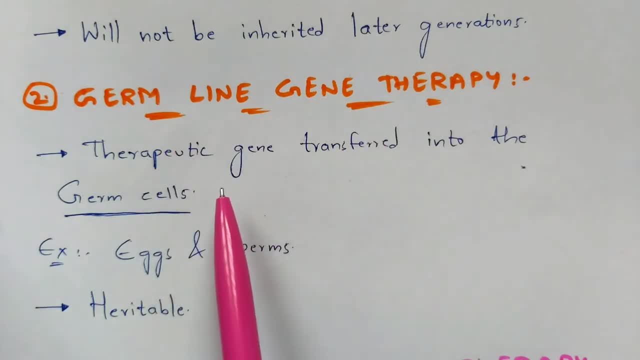 hence this process is called as germline gene therapy. so what are the examples of these germ cells like, let's say, eggs and sperms, right? so? as we are transferring this gene directly into the eggs and sperms, so it is heritable, so that it can, so that it cannot be that particular disease cannot. 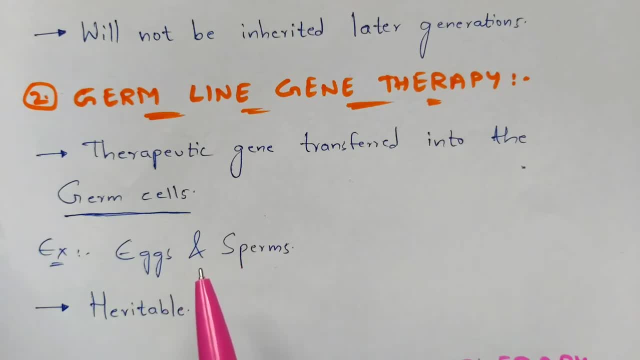 be passed to the future generations. we can also save the future generation people also. i mean our offspring and our children and their children. right, you can save your generations by the process of this germline gene therapy. hence it is heritable, because we are going to transfer the gene directly into the eggs and sperms. 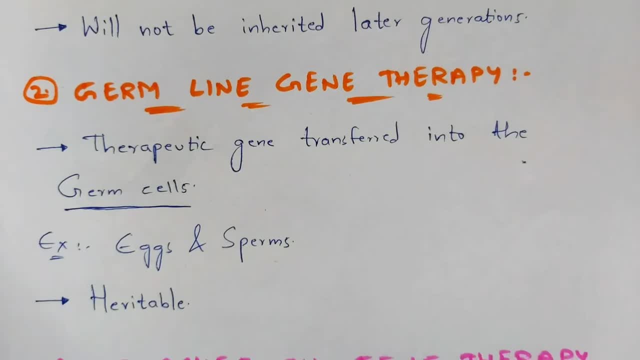 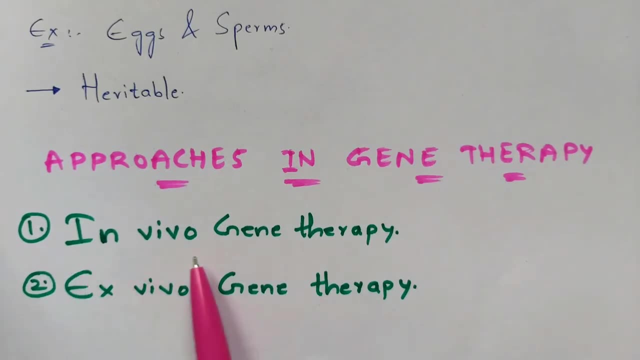 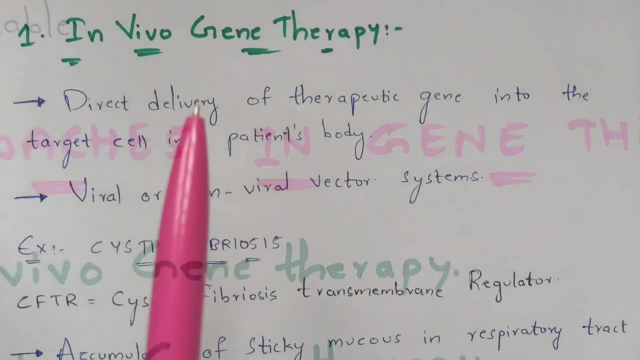 right. so these are the types of gene therapies and let us see what are the approaches in gene therapy. so there are two approaches in gene therapy. they are in vivo gene therapy and ex vivo gene therapy. so firstly, let us discuss about in vivo gene therapy. so, coming to the 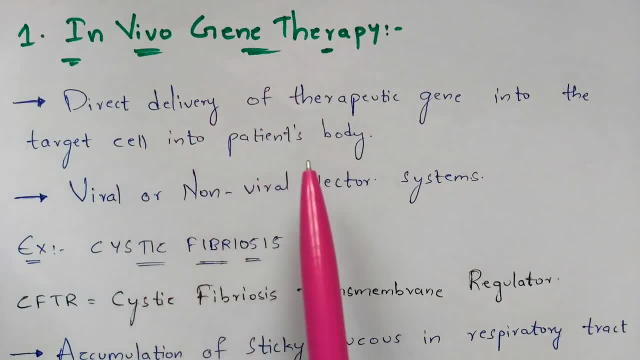 first one in vivo gene therapy. so the direct delivery of therapeutic gene into the target cell, into the patient body, is called as in vivo gene therapy. so what you mean by this statement? so here patient body is nothing but the person who is infected with this. uh, you know genetic. 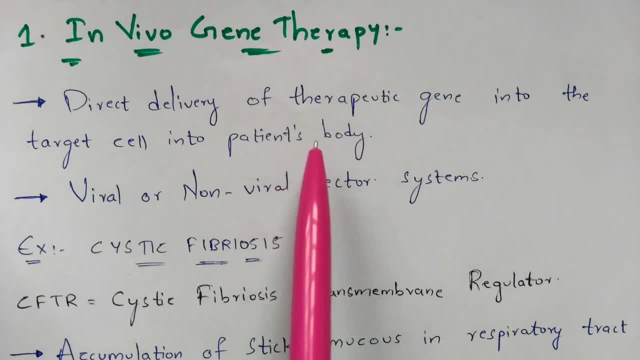 disorder. who is suffering with this genetic disorder- any type of genetic disorder is called as a patient- okay in this, in our case. so the direct delivery of therapeutic gene? therapeutic gene is nothing but a functioning gene, right, and the direct delivery of this functioning gene into the patient body there is. there is no. 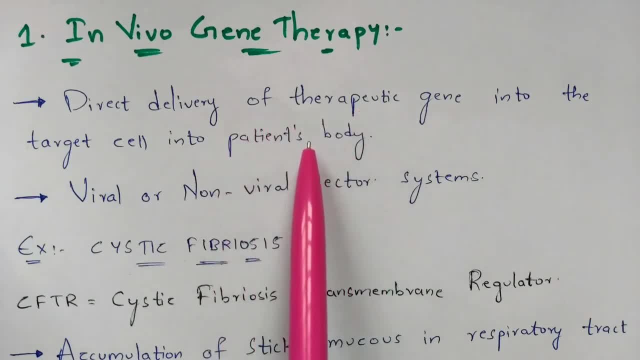 process involved just a. So the direct delivery of this therapeutic gene into the patient body will be done, Right, And that process, that direct delivery process, is called as in vivo gene therapy, Right. So a particular target cells will be selected in that or in that patient, and then that. 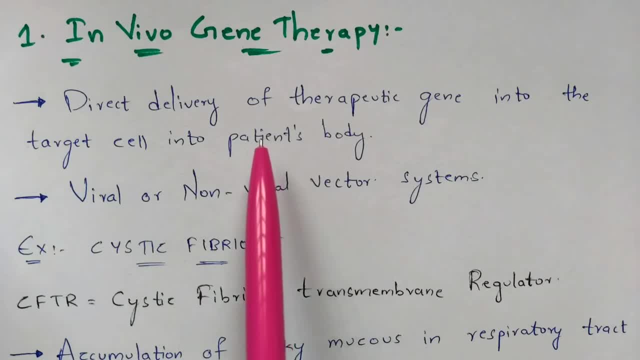 particular target cell will be selected right. So to the target cell. we are going to deliver that therapeutic gene Right, Directly. This is a direct process, Hence it is called as in vivo gene therapy here. in the process of this in vivo gene therapy- uh, not only in this in vivo, even in the, even in 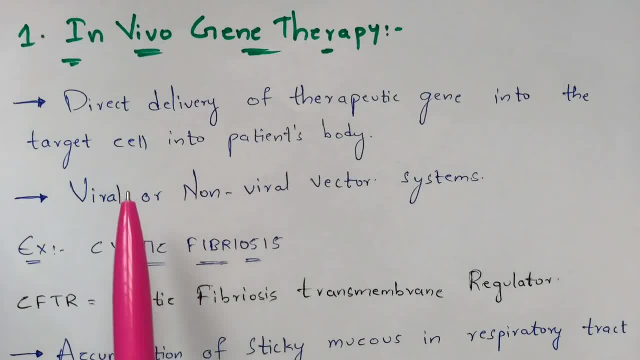 this second type, which is ex vivo gene therapy, vectors will be used. like there are two type of vectors. there are viral, are i mean viral vectors and non-viral vector systems. so in the process of this in vivo gene therapy, you can either use viral vectors or non-viral vectors. okay, so what are these? 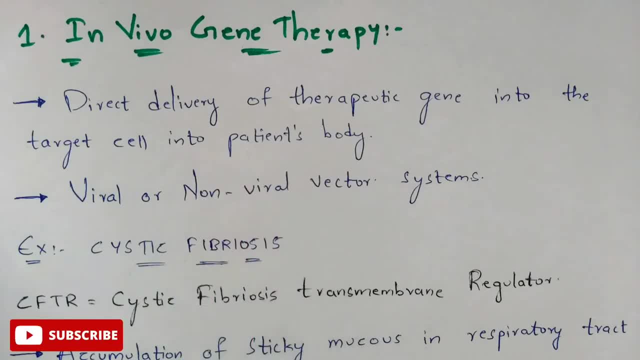 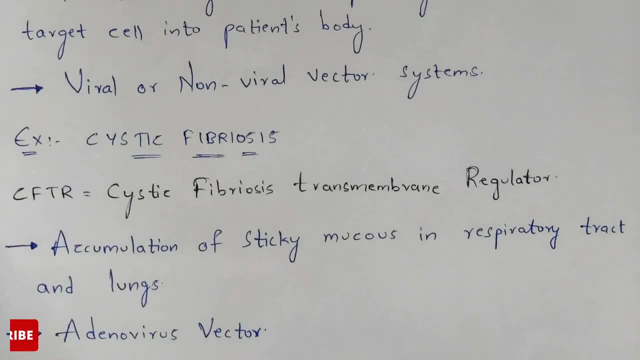 viral and non-viral vectors. i'm going to explain at the end of the video. okay, so the best example of this in vivo gene therapy is cystic fibriosis. so what do you mean by the cystic fibriosis? so cystic fibriosis is a disease, is a genetic disease which causes, you know, human beings. 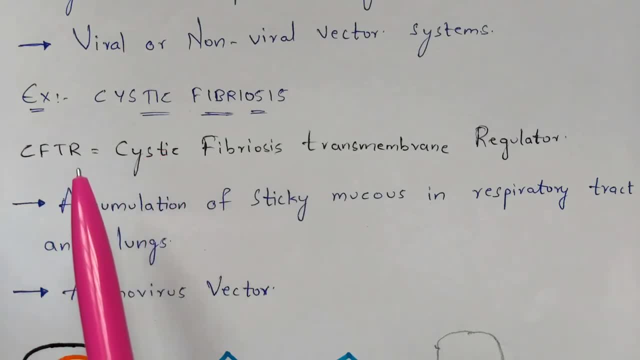 and i also explained about cystic fibriosis in detail in the diagrammatic form and the link will be provided in the description box. so if you want to learn more about this cystic fibriosis, you can watch that video. okay, so in this case of cystic fibriosis, there will be a lack of protein in that. 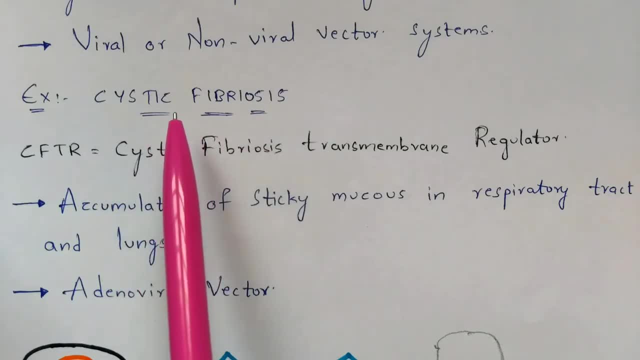 patient, hence he is infected with the cystic fibriosis. so what is that protein, or else what is the gene? that gene is called as cftr- it is abbreviated as cystic fibriosis transmembrane regulator. so there is absence of this cftr gene in the patient, hence he is suffering with a genetic disorder called a cystic. 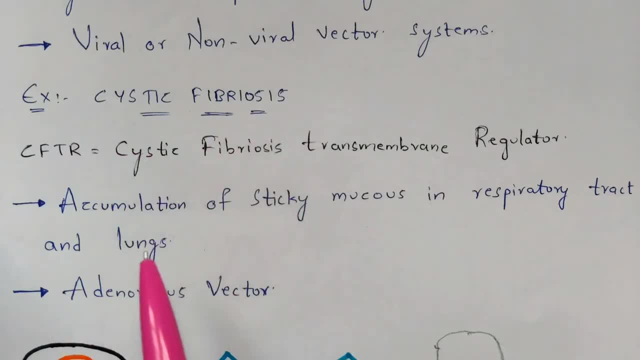 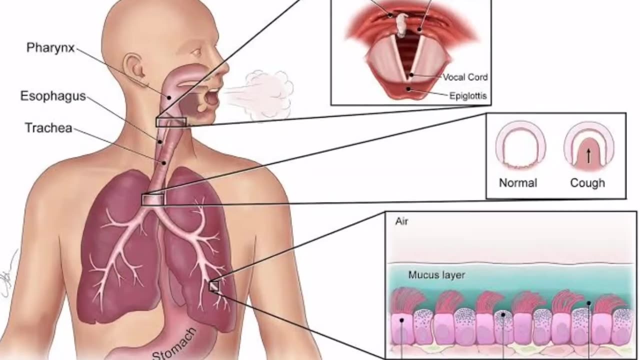 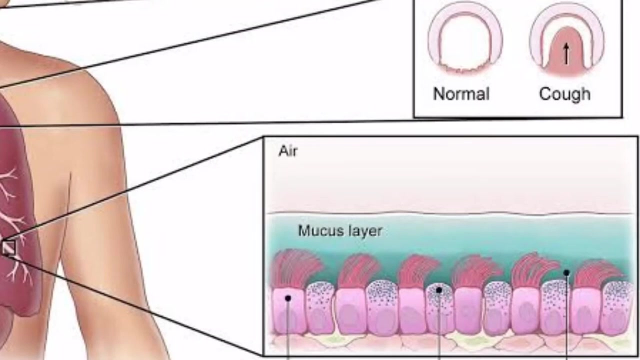 fibriosis. okay, so what is the? you know what are the symptoms which you can see once the person is infected with the cystic fibriosis. so what will happen? basically, there will be accumulation of sticky mucus in the respiratory tract and lungs of that human being, or as that. 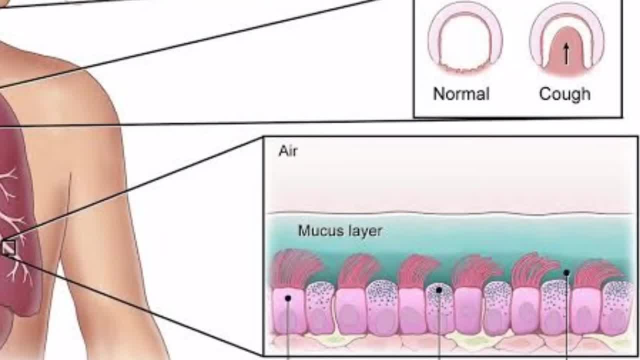 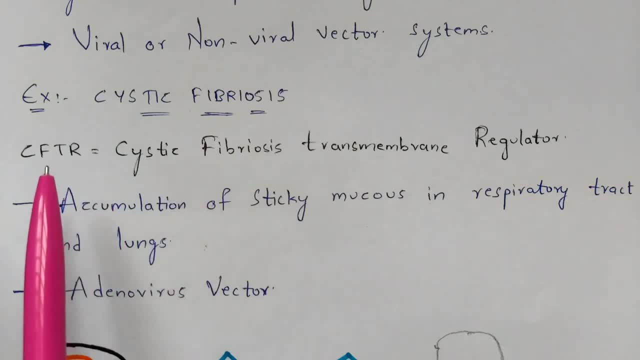 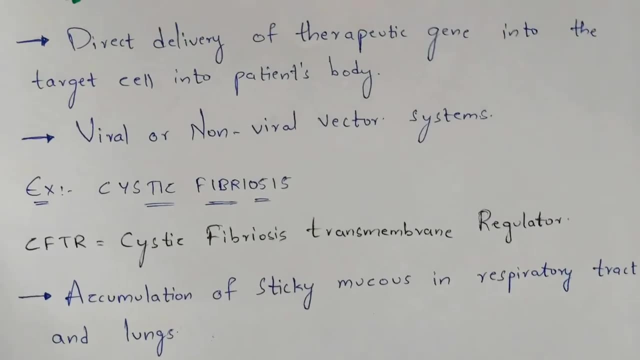 patient who is suffering with this cystic fibriosis genetic disorder. okay, so in order to cure this cystic fibriosis, we are going to insert this cftr gene by using a vector called as adenovirus vector. so already i have said you right. so in the process of this, in vivo gene therapy or x vivo gene therapy, 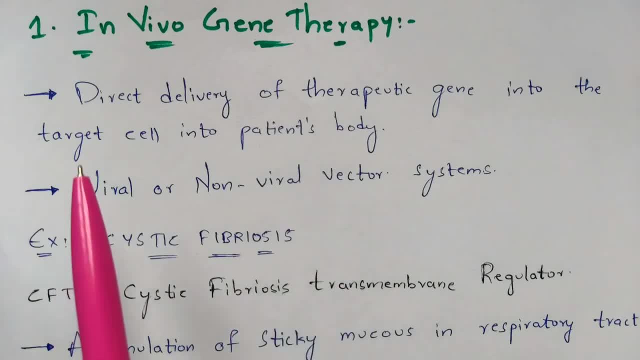 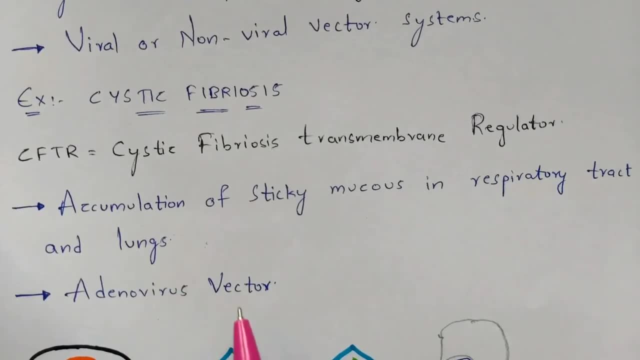 general, vectors will be definitely used. if the vectors are not used, then the gene therapy process cannot be done. this is very important to remember. so in the case of cystic fibriosis, here we are going to use adenovirus vector. so how the process will be, see i have clearly. 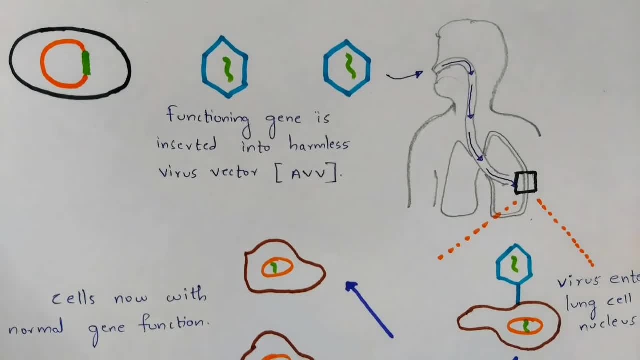 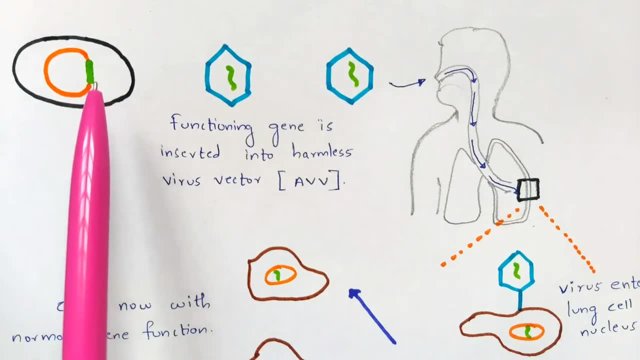 i am going to clearly explain in the diagrammatic form, so listen properly. okay, so now here. what we are going to do is that we are going to select a particular bacterium which is carrying the plasmid with cloned uh, normal human uh, this cftr gene. okay, let us go ahead and see. 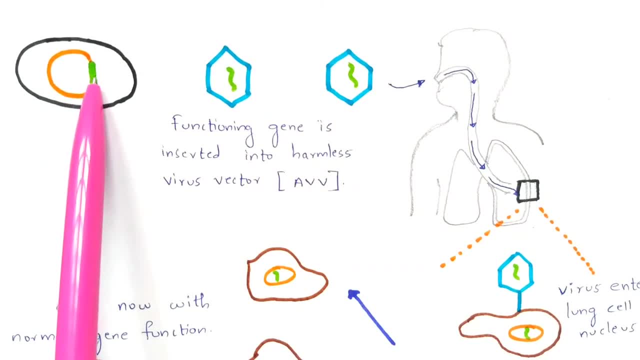 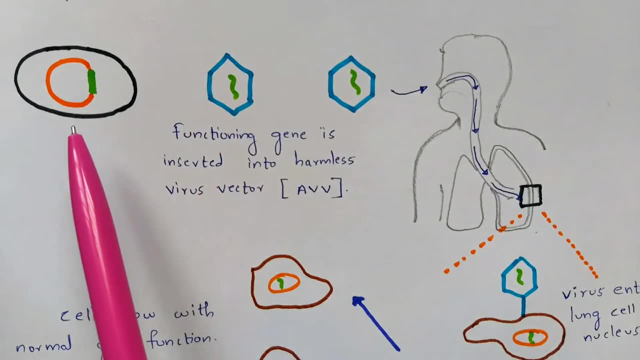 how it works. first of all, guys consider this green color. one is nothing but the cftr gene. okay, fine, so now the cftr gene. what you are going to do is that you, if you keep this cftr gene- i mean this bacteria i said you know you are going to select a genetically disabled retro. 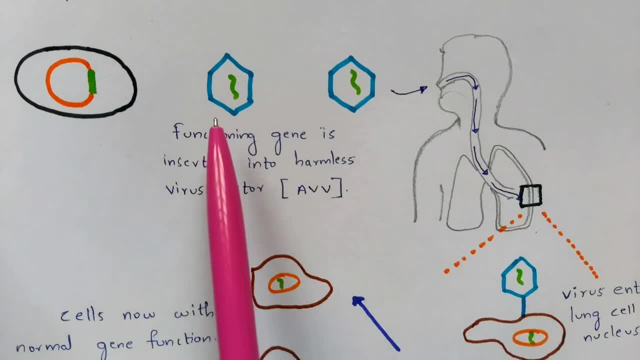 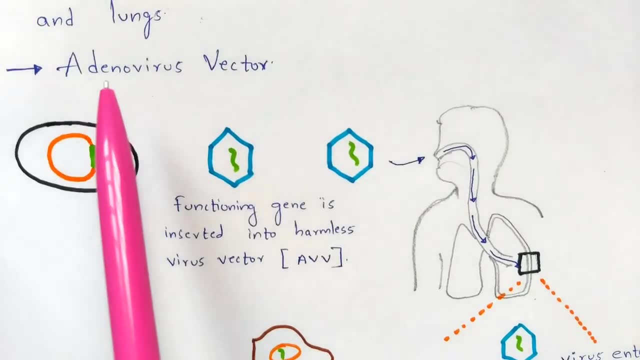 virus vector. okay, you are going to select a retrovirus vector. so, uh, you know what? here, in this case not retrovirus. here we have selected adenovirus previously, itself right, adenovirus vector. so now we are going to take that vector, i mean, which is adenovirus vector, which is 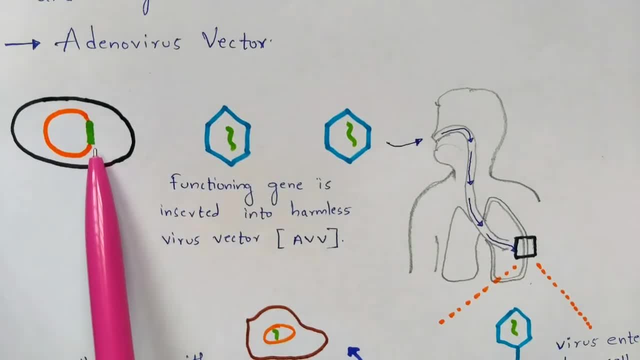 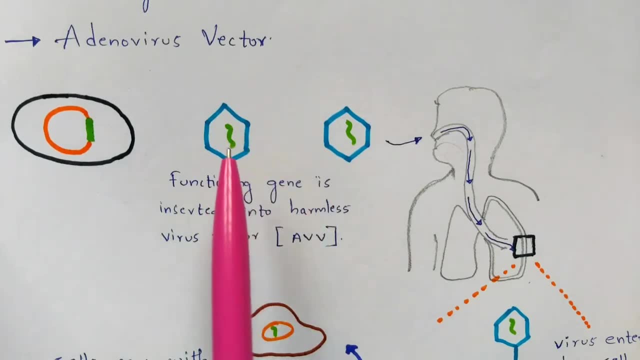 functioning gene is inserted. so this is functioning gene, right, and that will be inserted into this vector. okay, so remember, this is harmless virus vector, so as it doesn't contains any gene, right, this virus doesn't contain any gene, hence it is harmless, so as it doesn't contain any gene, so gene. 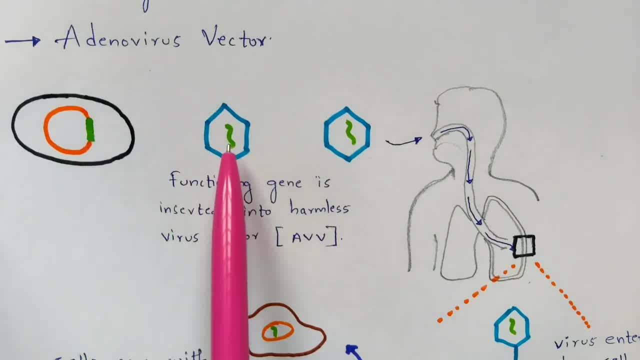 of our interest will be inserted into this harmless virus vector. so, in our case, what is harmless virus vector? adenovirus vector. okay, so now this functioning gene with adenovirus vector will be inhaled in, will be inhaled by the patient. either it may be given in the form of sprays or 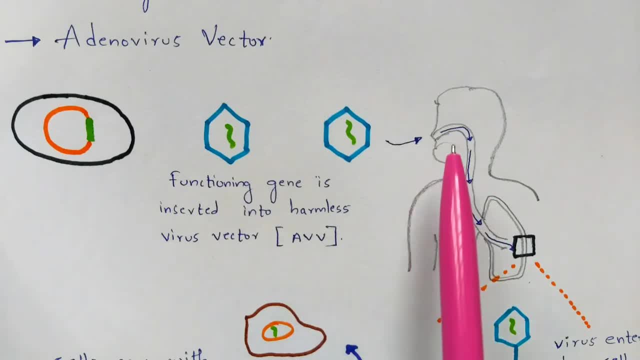 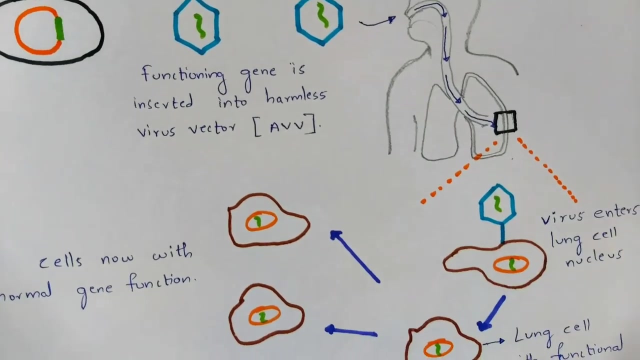 medicines. it will be inhaled by the patient. so once he inhale, what will happen then? this particular unit will enter into the membrane of the lungs. right, it will enter into the membrane of the lungs. so what will happen in the lungs, in the layer of the lung level? let us see clearly. so what will happen in the sense? so this: 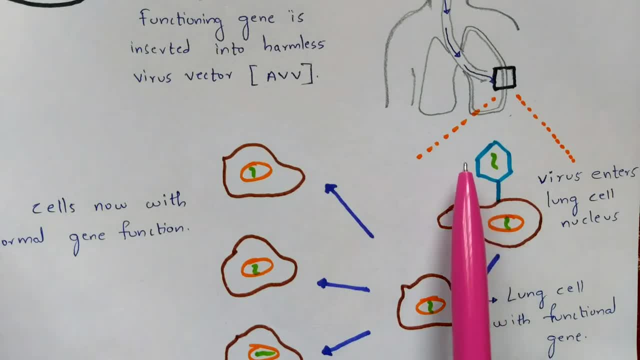 is a. you know what this is? a unit, unit in the sense the functional gene which is present in the harmless virus vector, which is called as adenovirus vector. so this is a unit. and now this unit is combined with this lung cells. so why this lung cells? because it has entered into the lung cells. 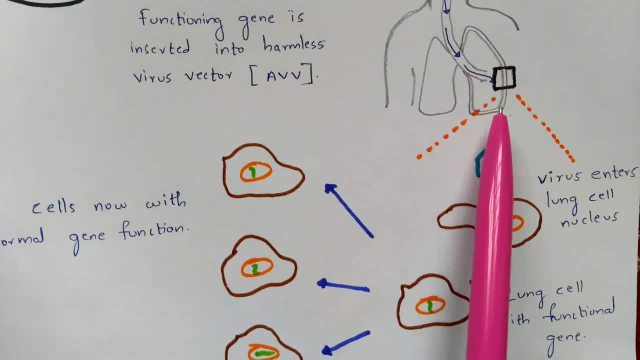 right. i mean, you know, the cell membrane of the lung contains lung cells, so it entered into the lung cells. so now, what will happen? now, this gene, now this gene which is present in the vector, will enter into the nucleus of the lung cell. and one more important thing which people have to 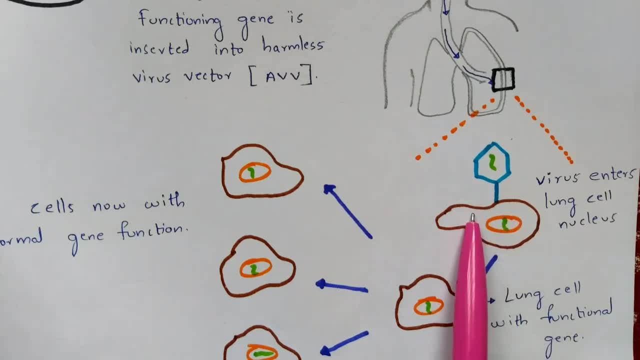 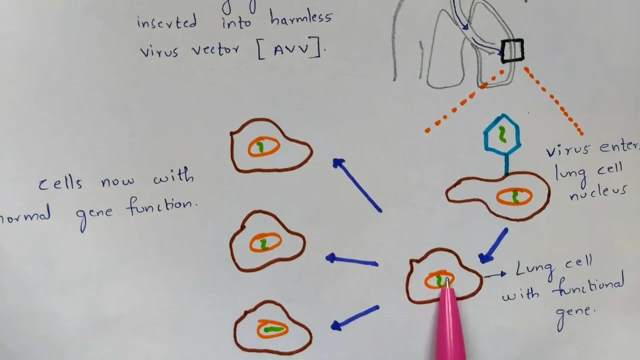 remember is that it will not directly enter into the nucleus. firstly, it will enter into the cell membrane of the lung cell, and once it entered into the cell membrane of the lung cell, then it will enter into the nucleus of that lung cell. okay, so, So now what will happen once it entered into the nucleus of the lung cell? now, this lung 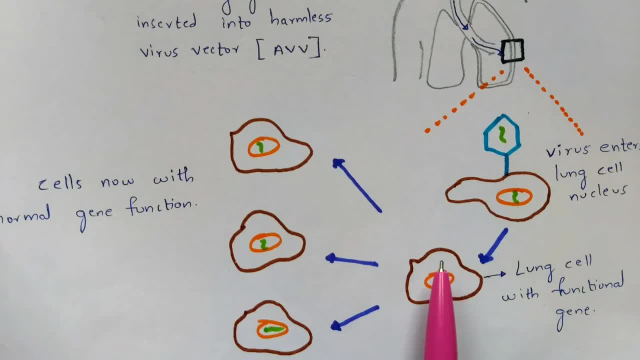 cell with functional gene will undergo the process of mitosis. Now what will happen Now? as it undergoes the process of division, it will get multiplied in number. So these are the cells now with normal gene function, which means it contains the gene. 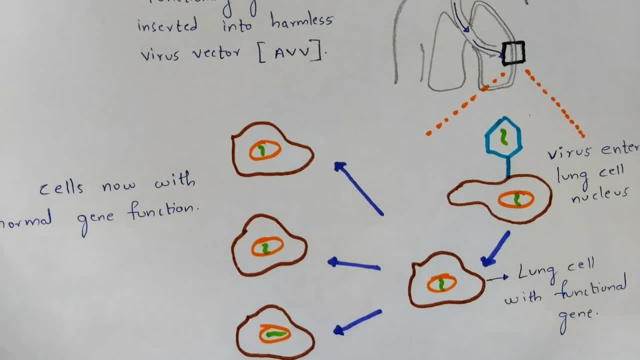 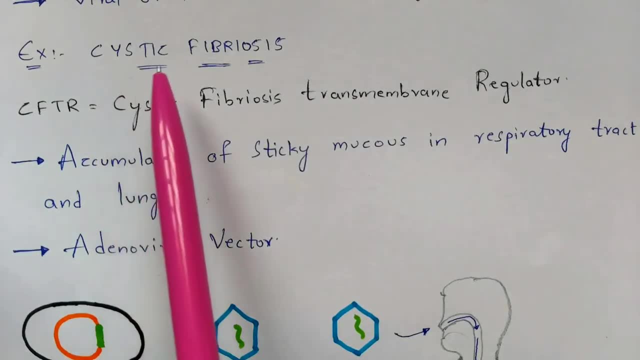 of CFTR, cystic fibrosis transmembrane regulator, which I have already said you So, as that patient doesn't contain this CFTR gene, hence he is suffering with cystic fibrosis disease, So now we have inserted CFTR gene artificially by the process of this gene therapy. 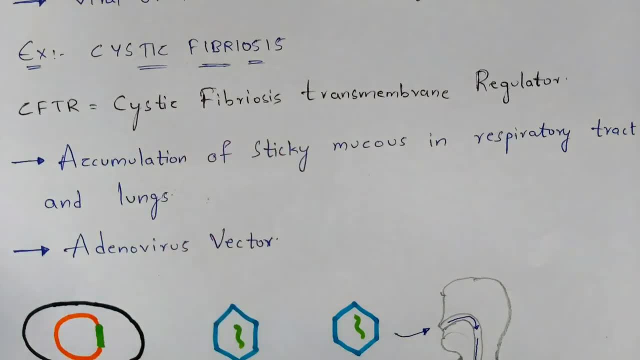 Now there will be no more cystic fibrosis disease which you can see in that patient, because we have cured that patient with this in vivo gene therapy process, right? So this is what about in vivo gene therapy. Now I'm going to explain about ex vivo gene therapy. 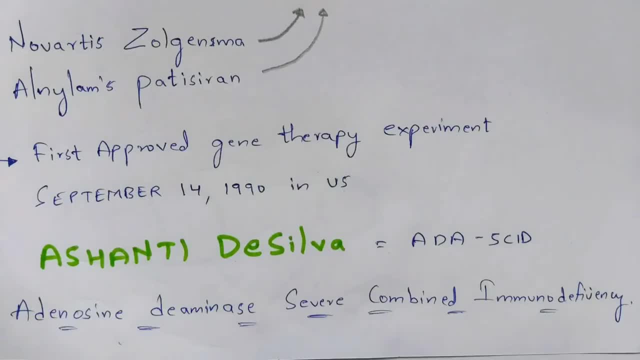 So now let us discuss about ex vivo gene therapy. So previously beginning itself, I have said you right. There is a patient called us Aashanti Desilva, who is four years old, and she is suffering with this ADS KIT disease. I mean adenosine D-aminase, severe combined immunodeficiency. 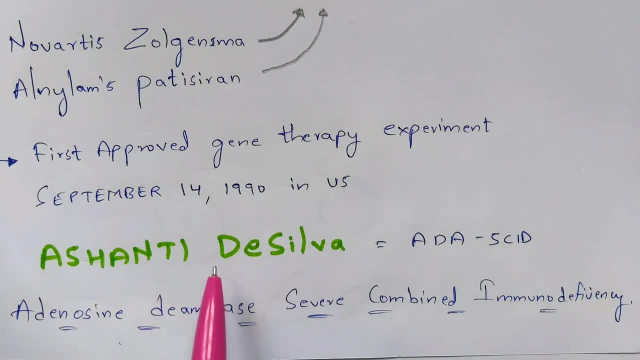 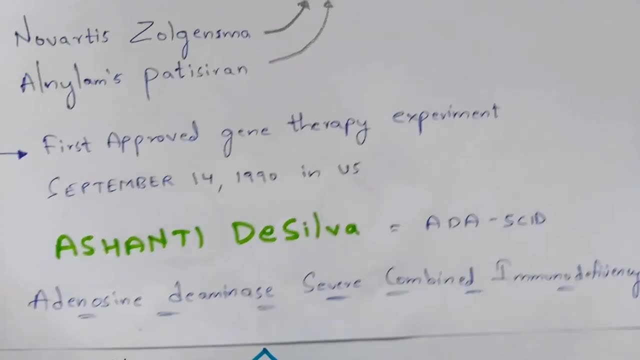 and now we are going to take the example of this patient itself for our ex vivo gene therapy process. So remember that this is ADS KIT, which is adenosine D-aminase- severe combined immunodeficiency. So now the disease will be: uh, the disease can be seen in that patient due to the lack 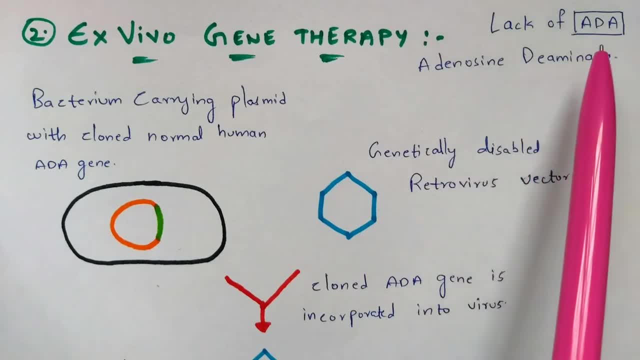 of a gene called as, or is due to the lack of an enzyme called as a da. so what is this? a da, adenosine da minus. okay, so when there is a lack of this enzyme, then that person will be infected or else will be suffered with that genetic. 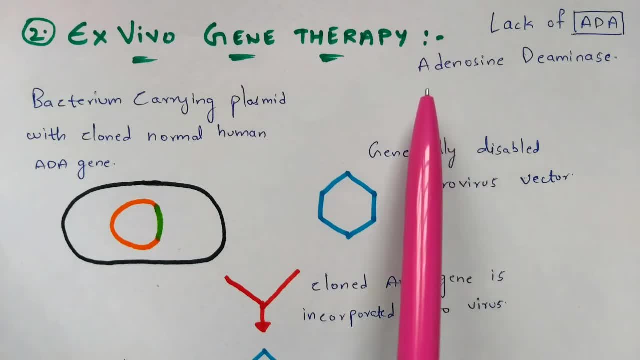 disorder which is called as a da skid. so now, if that patient is suffering with that disease, then how we are going to cure? we are going to cure by the process of ex vivo gene therapy. now I am going to explain the process of this ex vivo. 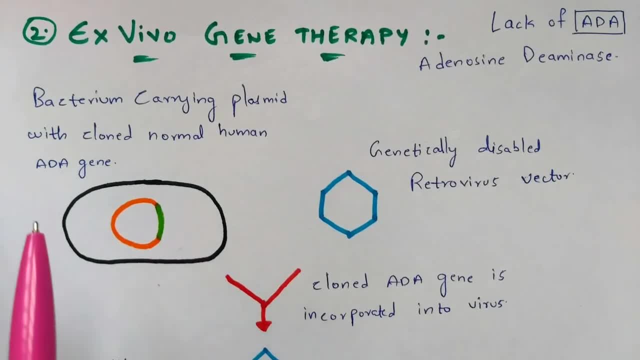 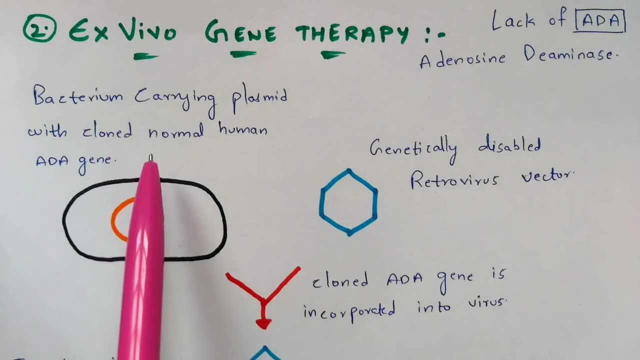 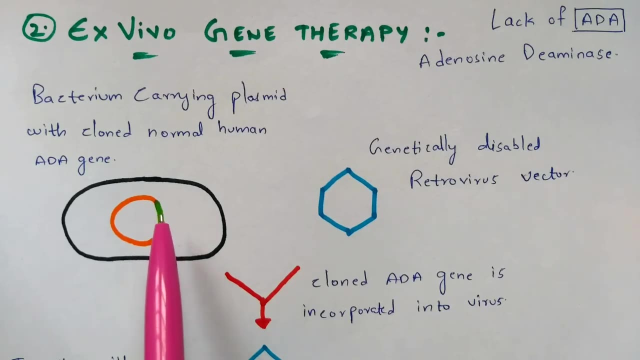 gene therapy diagrammatically. so listen properly. so now what you are going to do is that you are going to choose a particular bacteria which is carrying plasmid with cloned normal human a da gene. so this green color one which I have drawn is nothing but the a da gene. okay, so this a da gene is responsible in. 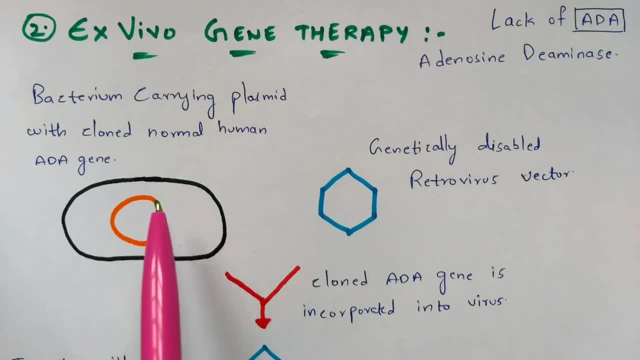 order to cure that genetic disorder. so if you keep this aside and now you are going to choose a genetically disabled retrovirus vector, so previously what we have chosen is that we are going to choose a gene which is called as a da vector and also summarized it with adenosine duodenum. so in the case of 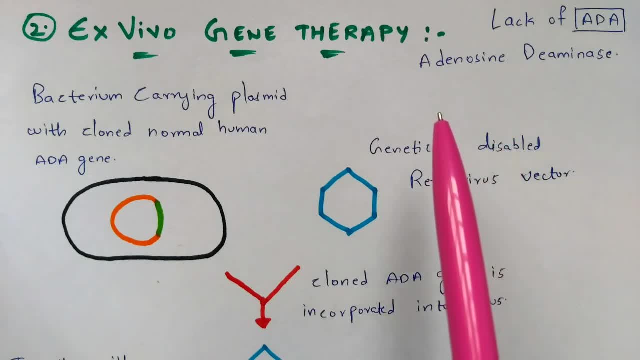 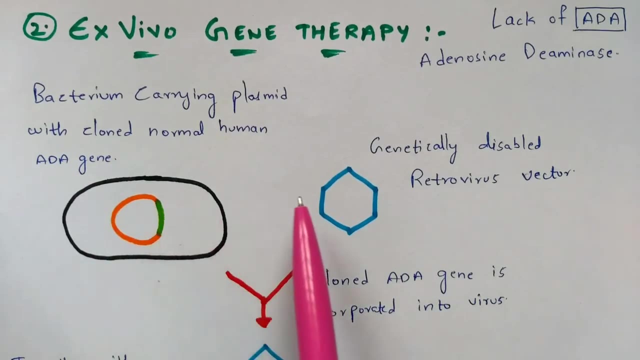 LV o gene therapy. what we have chosen? we have chosen adenovirus vector. but now here, what you are going to choose. we are going to choose retrovirus vector, right, but but different type of genetic disorders. we are going to use different type of vectors. okay, either it may be viral vector of non viral vector. 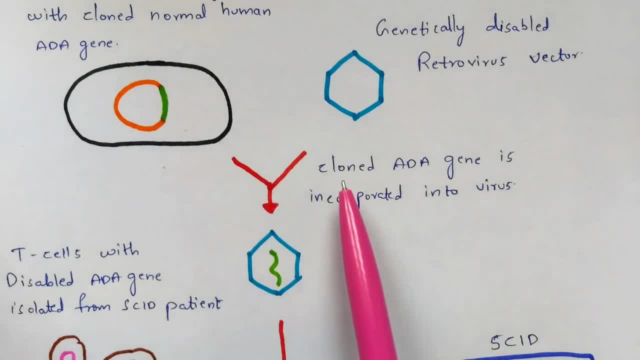 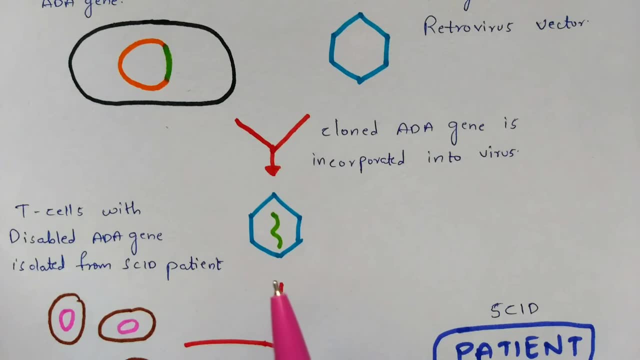 okay, so now we have them. so cloned ada gene is incorporated into virus. okay, so this is harmless virus before itself. i have said you: this is harmless virus because it doesn't contain any genetic material. so, as i have, as i have shown you, that does this contains any genetic material. no, right, so we are inserting the. 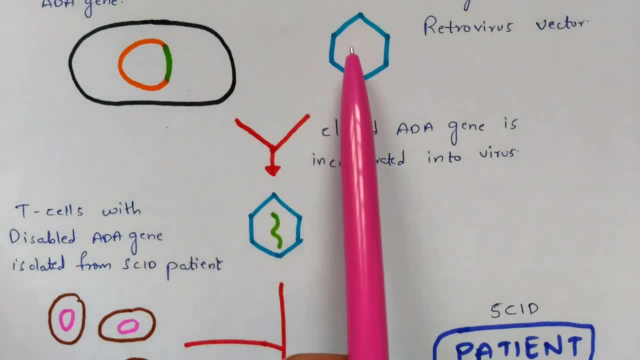 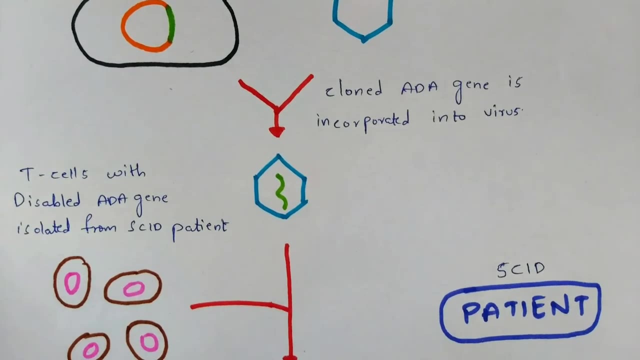 we are inserting the pure artificial gene into this virus, but this doesn't own a genetic material, right hence now, this is harmless. so now, ada gene has been inserted into the retrovirus vector over here and now, on the other hand, what you're going to do is that you're going to isolate t cells with 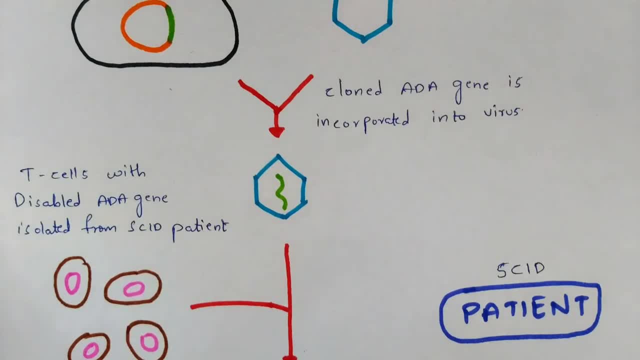 the disabled, ada gene from the skid patient. skid patient in the sense, i mean the person who is infected with this, uh, you know, ada skid disorder. i mean from that patient which i have said, you right, from that patient who is four years old, uh, as he, as she, is suffering from skid. 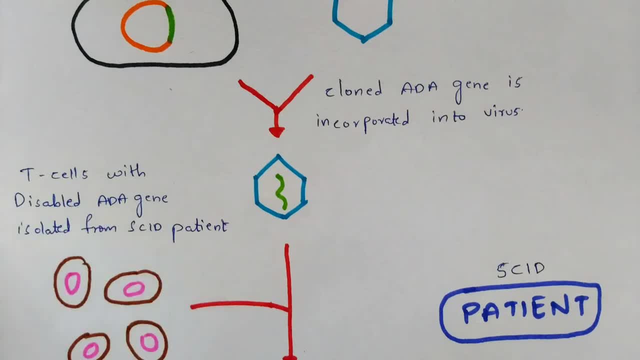 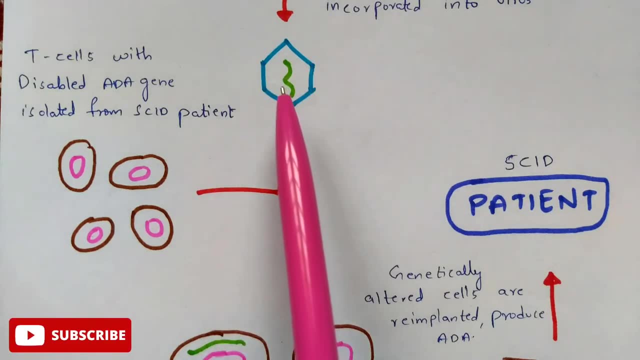 you know from that patient, who is 4 years old, as she is suffering from skid. Now what you are going to do, you are going to isolate T cells from her. Once the T cells is isolated from her, then what you are going to do: you are going to introduce this incorporated virus vector into this. I mean onto this, not into onto onto this T cells. 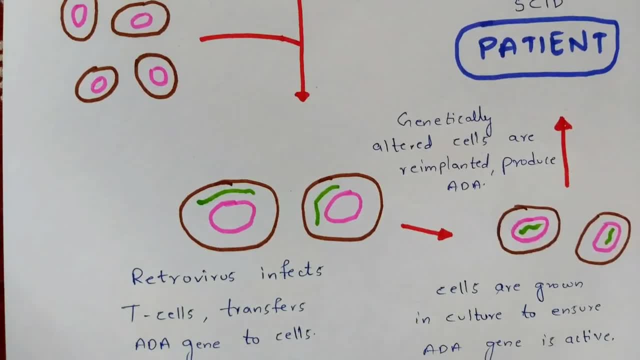 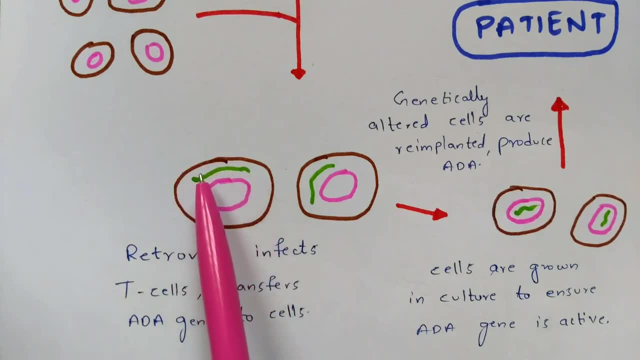 Now, what will happen? Now that ADA gene will enter into the cell membrane, not directly into the nucleus, which I have said you, it will enter into the cell membrane of the, of the, you know, T cells, right? 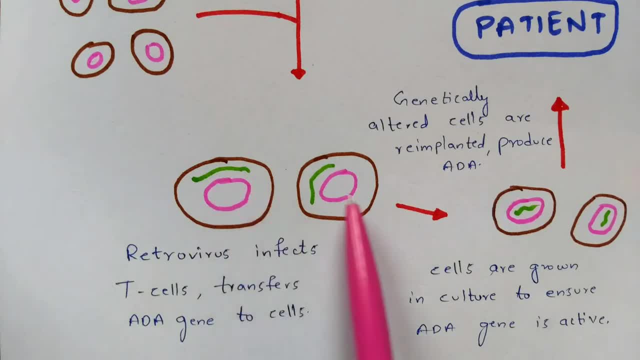 And now, once it entered into the cell membrane of this T cells, then later it will enter into the- you know what- this nucleus of the T cells, right? So once they are entered into the nucleus of this T cells, then they will be cultured. 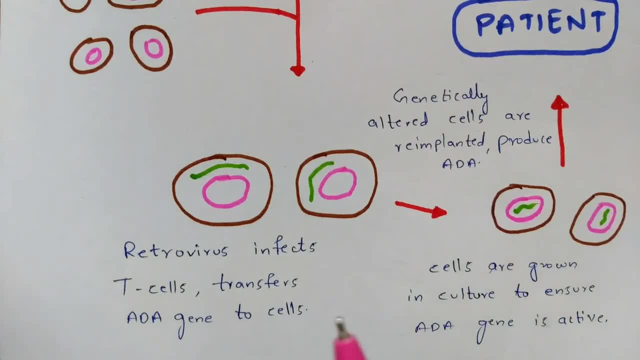 So how the culture process will be, I have said you right. So if you see my previous videos, I have explained you about cell culture process detailing, and the link will be provided in the description box. So once the culturing process will be done in such a way that you are going to take a petri dish and in that petri dish you are going to place these two cells, or else any one of the cell will also be no worries over there. you can take two cells or any, or any of the cell, okay. 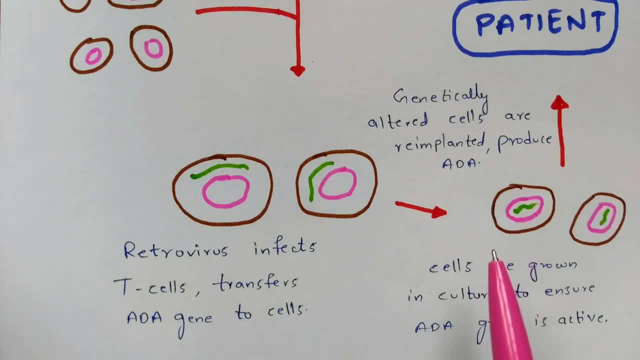 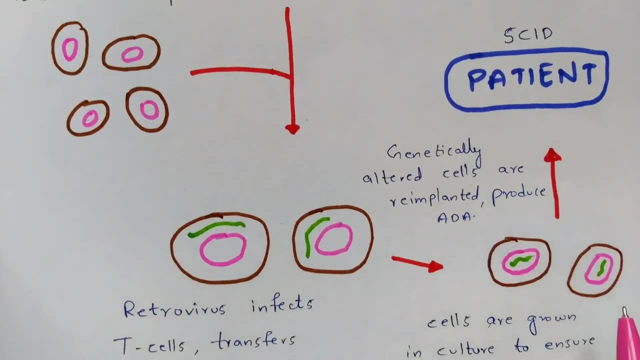 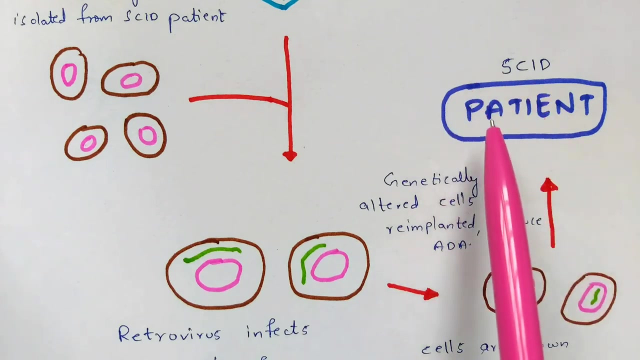 So you are going to place that cell in the petri dish and you are going to add the nutrients for that. So by absorbing the nutrients, these cells, we know it will get Proliferated, which means it will get divided by the process of mitosis, by using that nutrients which we have added. So once the once it utilizes the nutrients, then what will happen? Then it will get proliferated and that will be implanted into the patient who is suffering with SCID disorder. So here the patient, in the sense, the. you know the name, the. I have said you her name, right? 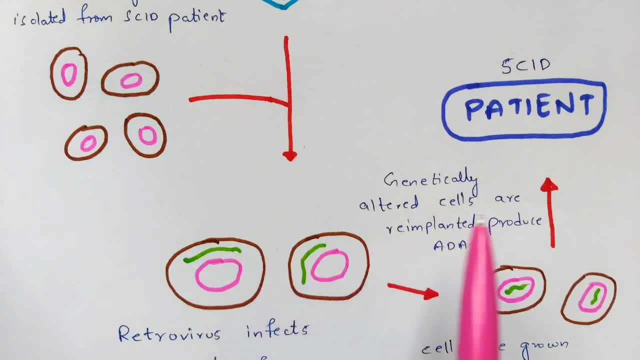 Ashanti Disilva, who is suffering with ADS, kid and and now this: the proliferated cells, the culture cells will be implanted into her, who is four years old, right And now. once they are implanted, then she will not be suffered with this disease anymore because we have cured the disease by the process of XVV gene therapy, right. 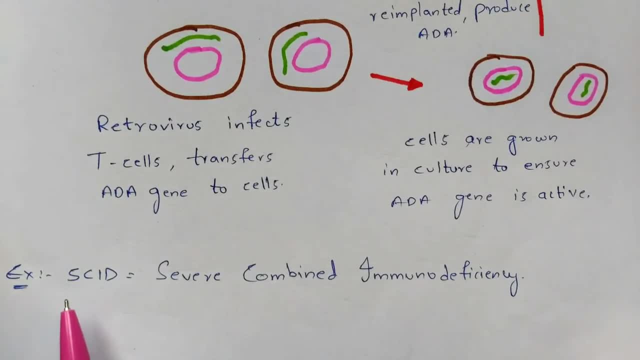 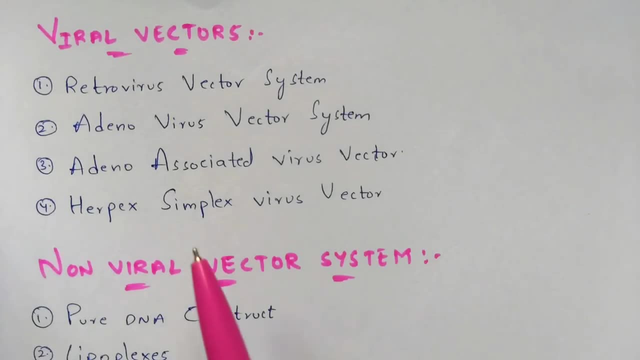 So here, the best example which we have chosen for our interest is SCID, which is CVO, combined immunity deficiency. So I already said you right For the process of this gene therapy, either it may be in vivo gene therapy or XYV gene therapy. 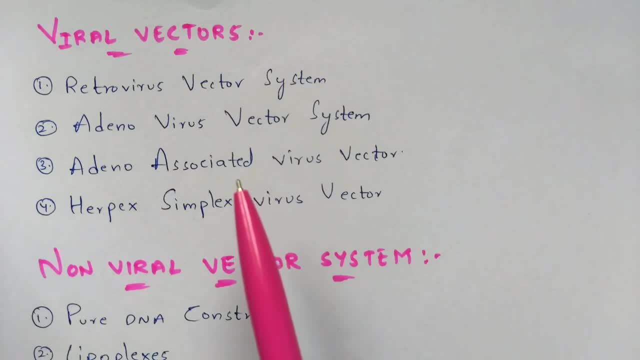 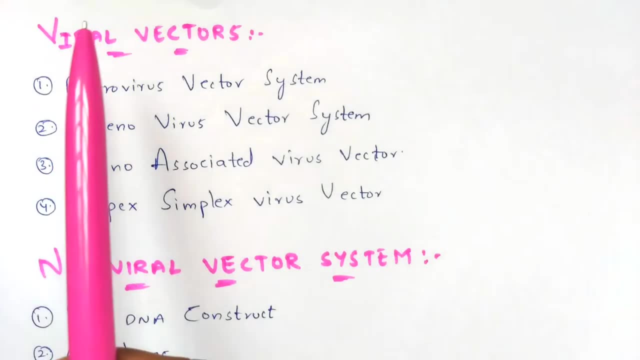 viral vectors or non-viral vectors are definitely used. so the best examples of viral and non-viral vectors i have- i have researched a lot and i have got their names. like in the case of viral vectors: retrovirus vector system. adenovirus vector system. adeno associated virus vector herpex.